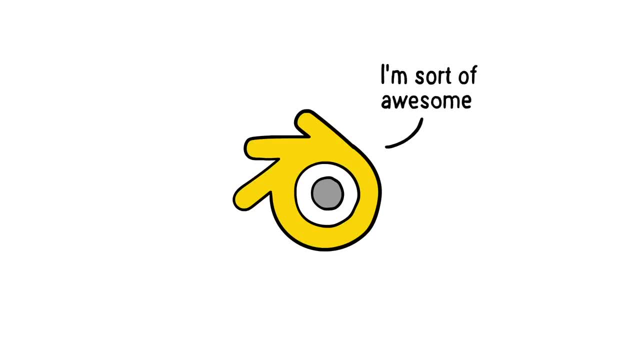 but I'm going to be mainly focusing here on 2D animation apps. If you want a nice 3D app, just leave now. Go Check out Blender. That's where you want to be looking. So a list. I made a list. These are the things that I'm looking for in an app that. 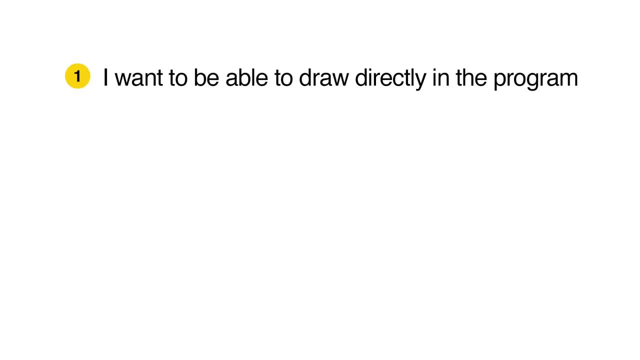 can replace Animate for me. One: I want to be able to draw directly in the program and draw fairly well. Two, I need to be able to import sound so I can do things like lip-syncing, also timing my animation to what's happening in the video. Three, I would like a symbol library. 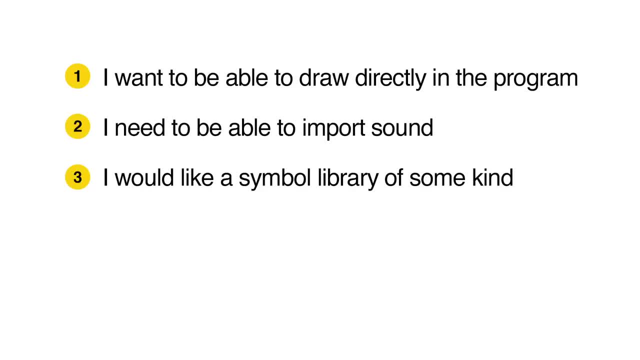 of some kind or some shortcut so I can reuse assets that I illustrated in one part of the video later on in the same video. Four, a timeline that lets me tween. Basically, tweening is when you move an object from, like one place to another place and then you move. 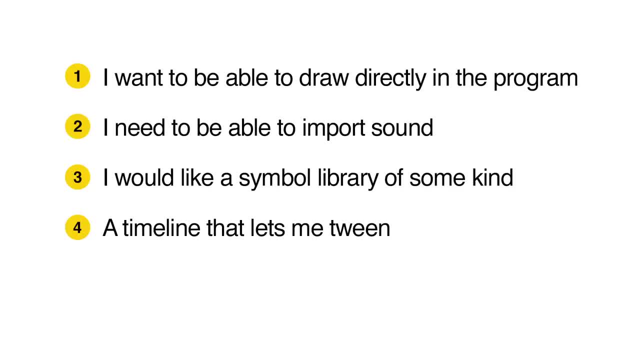 it from one place to another or zoom in and out, And what the program does is it handles all the frames in between, hence the term tween And five. it has to be free. None of this free trial stuff or in-app purchases- Free as in. I have some extra cats here. You can have one for. 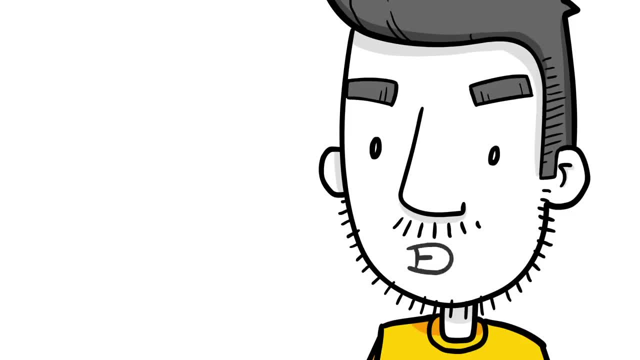 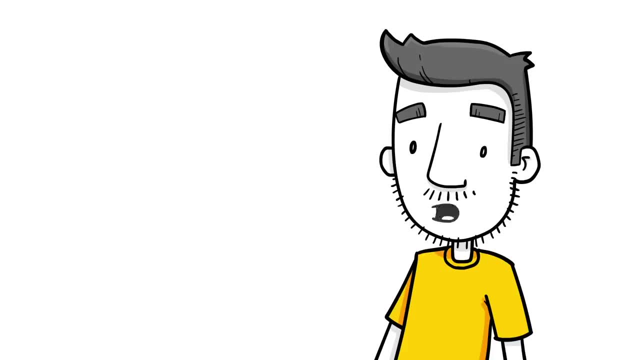 free, Free. I'm not a fool. I don't pay for cats. So those are the big things. Not every app here on this list has all five of those, but if I can get most of the way there, or if I think they're. 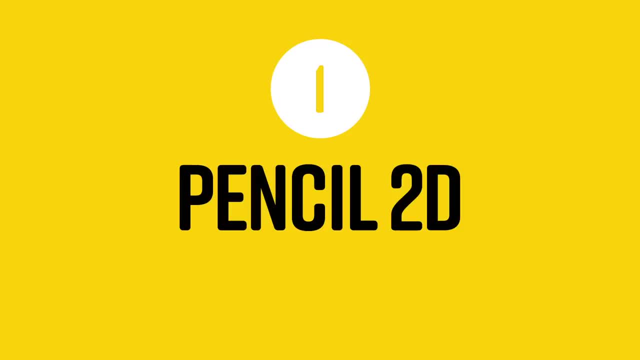 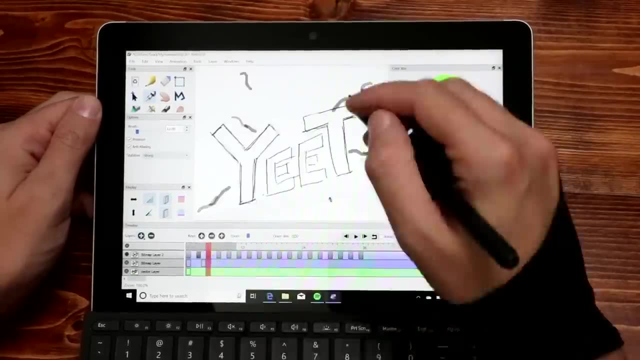 interesting enough, they made it onto this list. Alright, so let's get on with this First: Pencil 2D. It's an open-source 2D animation program named after pencils. It has a lot of the features that I'm looking for, but not quite. 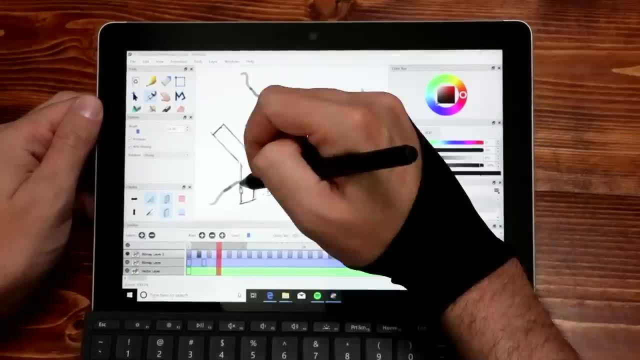 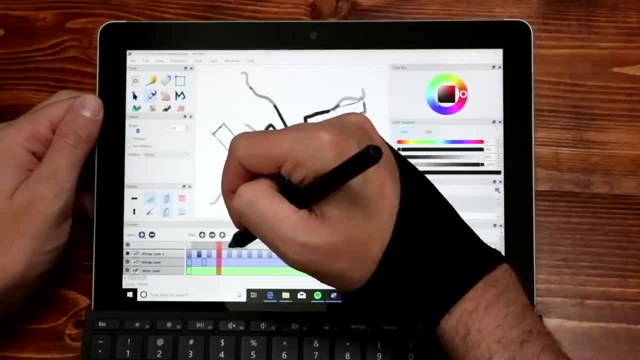 everything It has: raster and vector tools. Vector drawing tools is something that Animate has as well. If you create a vector asset and you need to zoom in on it, say in a future scene, you can scale it up, No problemo. You try to do that with raster graphics, it's yes problemo. They got all. 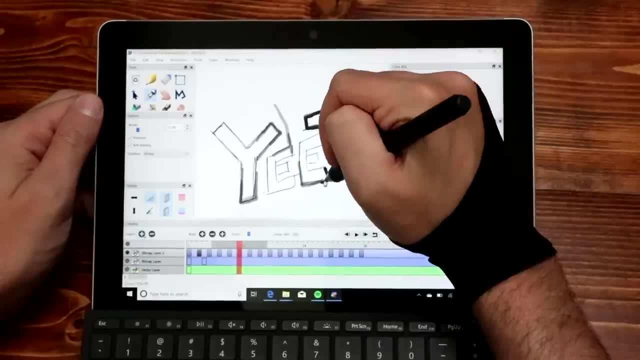 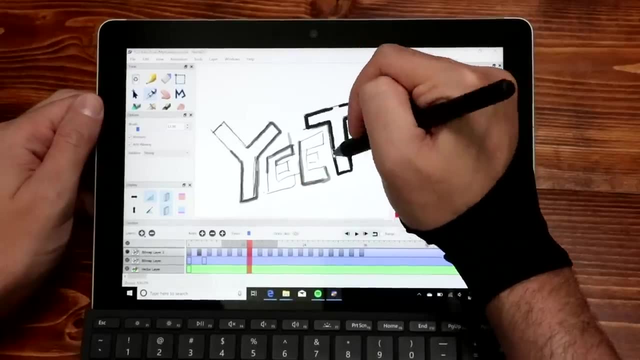 blurry and fuzzy and gross, So I like working with vectors in animation so I can reuse the art assets where I can. Some of the other apps on this list can be overwhelming, especially in the first day or two when you're using them. I didn't get that feel at all from Pencil 2D. This is. 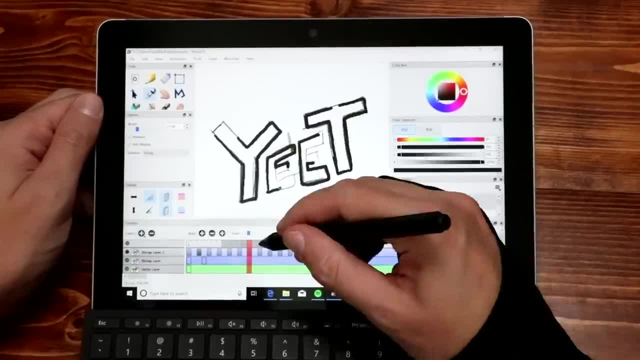 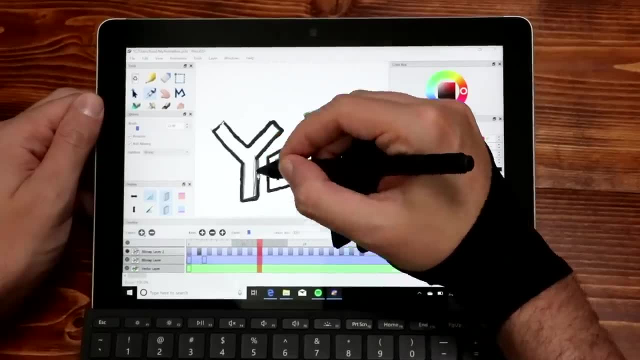 definitely one of the, if not the most, user-friendly apps on this list And because of that it can feel a little limiting at times. I know the drawing tools definitely felt limiting to me. You just can't do all that much. The timeline is also really simple, but if you're. 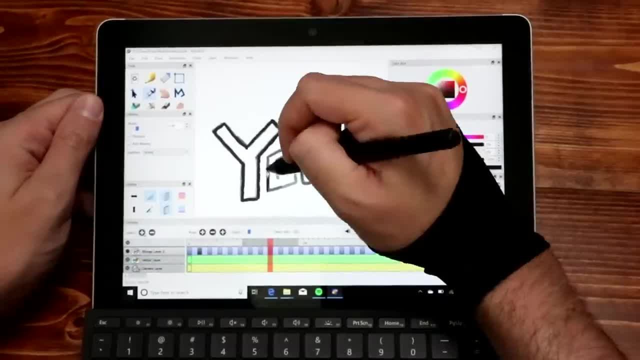 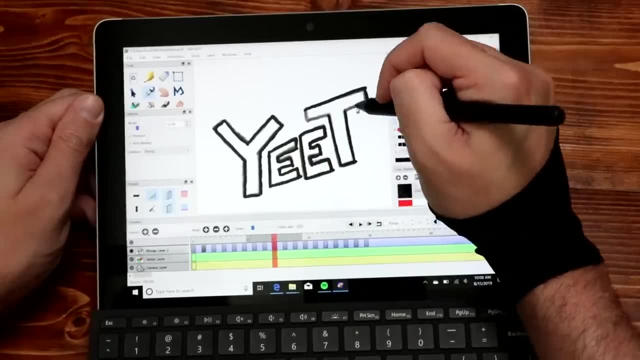 just starting out. that's not necessarily a bad thing, since a lot of animation apps can seem overwhelming, especially when you dive into the timeline and everything that can be used there. Overall, Pencil 2D doesn't exactly fit my needs. The vector tools are a nice touch, though I'd 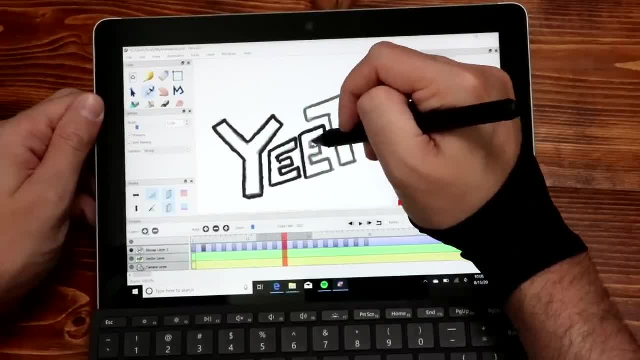 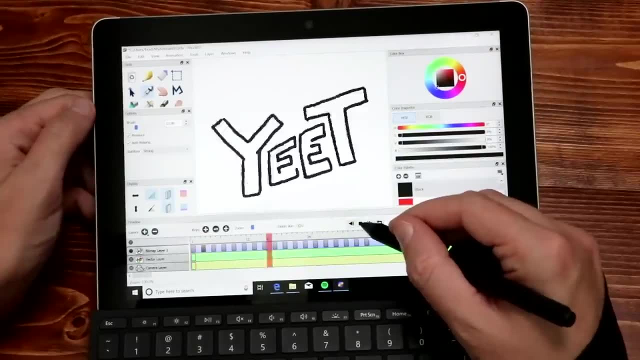 still like to have symbols and I'd still like to have tweening or something that would let me work with this application in the same way, but I still thought it was good enough to make this list. It's available on Mac, Windows and Linux. However, I would say when I first tested it out on the Mac, 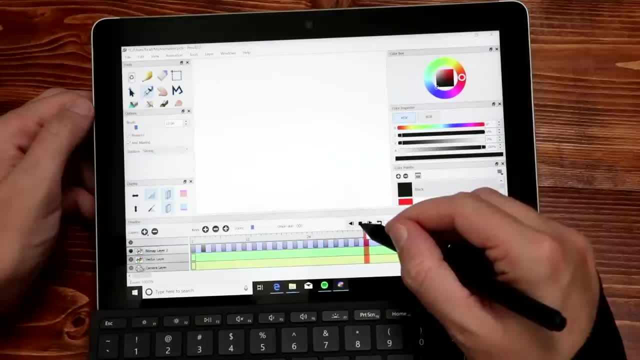 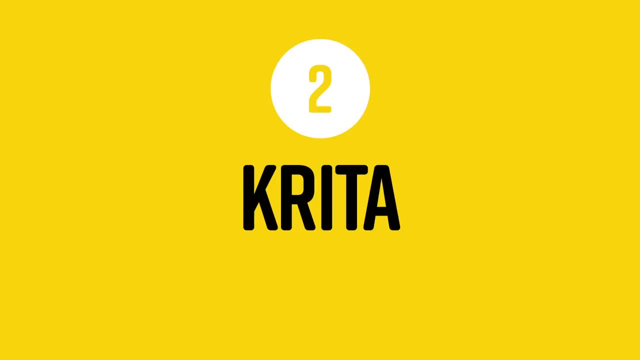 I would recommend using it there. It's a little wonky. especially when I was painting, The brush drag was really slow and it can be kind of buggy. Okay, it could be very, very buggy. Next up on my list is Krita. Krita also made my other list of favorite free drawing apps that I 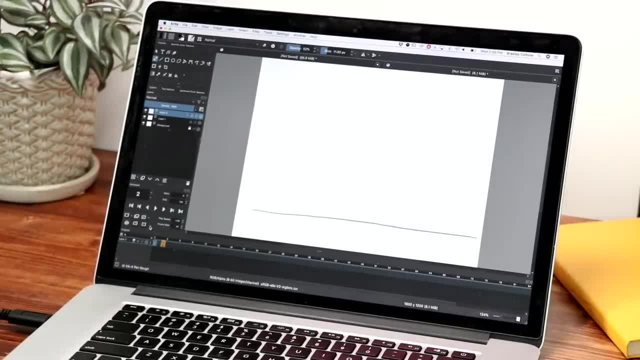 made a couple weeks ago. Actually, Krita is my favorite free drawing app. Since Krita is a full blown art app, I expected the animation features just to be kind of bolted on as an afterthought. but what really surprised me as I dug in is how. 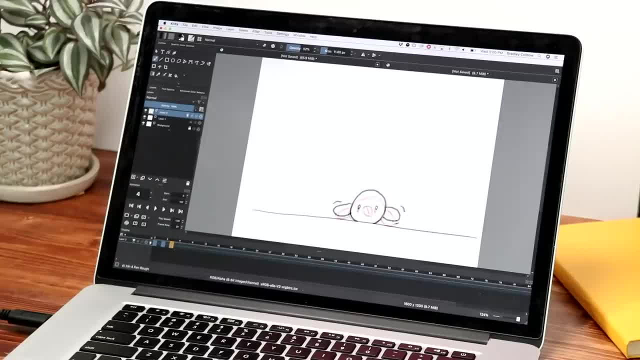 well thought out they are. If you go into the workspaces, change it up to animation, you'll get all the tools you need to get started: Adding frames, onion skidding, frame rate, adjusting- all of the essentials right there. It doesn't have symbols. 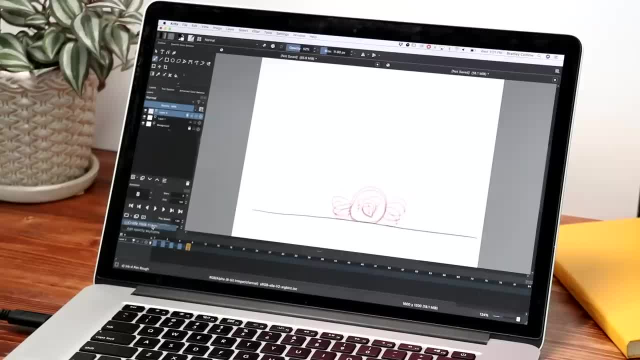 it doesn't have tweening and at this point it doesn't perfectly fit my workflow, but you can pull in audio files And the big benefit, one big benefit that Krita has over something like Adobe Animate is the depth of the painting and drawing tools at your disposal. 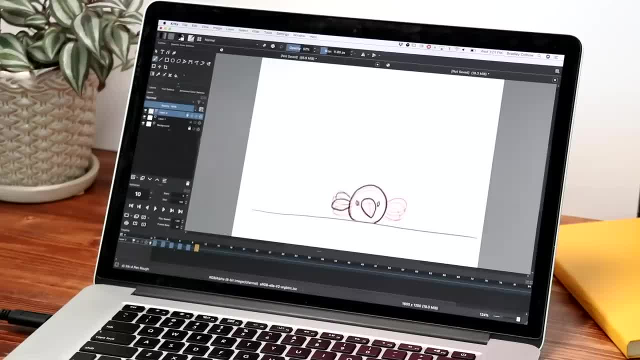 so you don't have to worry too much about the depth of the painting. In Krita, you can pretty much paint in any style that your heart desires: Paint brushes, textures- everything that you can paint with in Krita when you're just drawing and painting around, 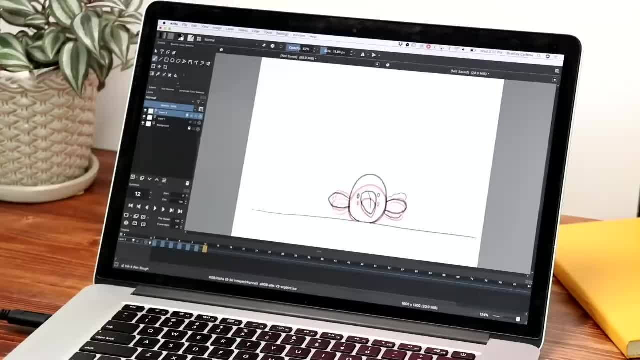 are at your disposal for animation as well, But what I really like here is the frame by frame interface. Let's take a look at some of the streamlined UI tweaks they make to make this fun to animate in. The first is something called the auto frame mode When it's turned on. 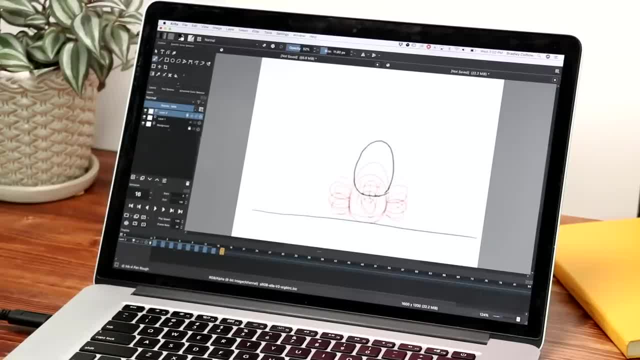 you start to draw on a new frame, It'll just make a new frame and it'll just make a new frame. You don't have to right click and say, make a new frame and then name it. All you have to do. 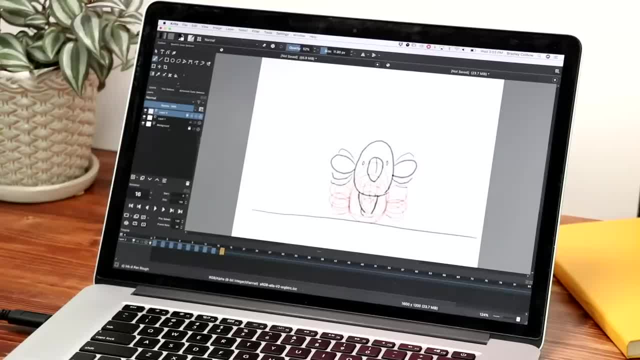 is click on the next frame, start drawing, and it's going to automatically keep what's in the previous frame that came before it. And as I'm describing this, I'm realizing this sounds really boring, but the reason I like it so much is because it cuts out so many extra steps, as you. 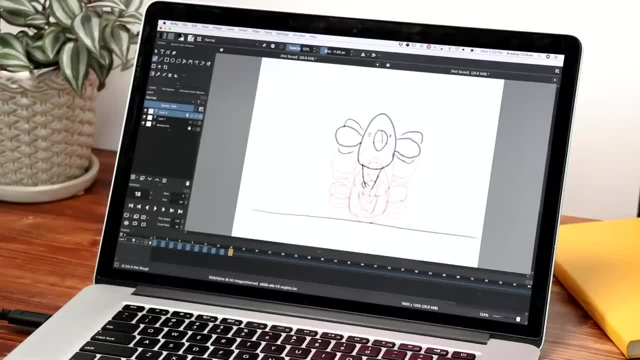 go. When you create hundreds of frames, when you're doing an animation, all those extra little clicks add up. You can tell that this was thought through by someone who's done a fair amount of animation for at least one or two years, and they're still doing it, and they're still doing it. 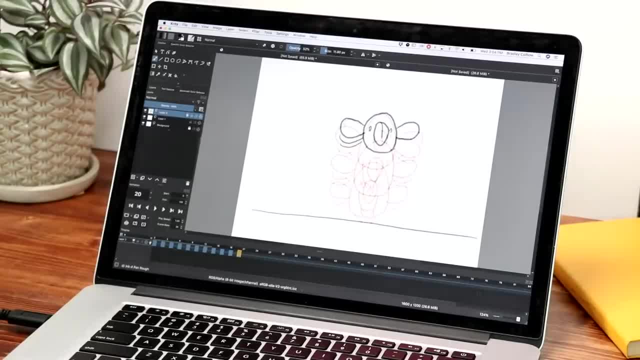 It's frame by frame animation in the past and understands the process and the workflow. As an extension of this nice workflow is the ability to set up keyboard shortcuts so you can quickly set up the program to work the way that you need it to work And if you're using a drawing, 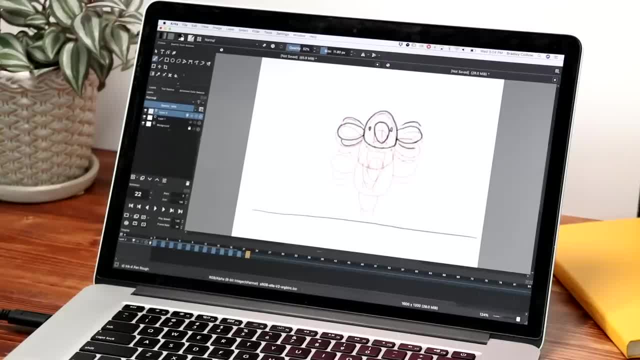 tablet with hotkeys you can map those shortcuts that you just put together to your drawing tablet and make your life even easier. You do need a plugin to export your videos, but once that's set up it's pretty easy to use. I did say in one of my videos a couple weeks ago that I was 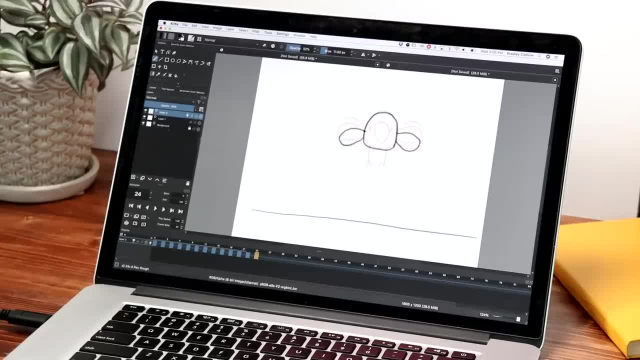 thinking about doing a tutorial on how to use a drawing tablet. I did say in one of my videos a tutorial on how to use a drawing tablet to can put together, So I'll stick the link down below in the description. So Krita is free if you download it from their website. I heard it's also in the Windows Store. 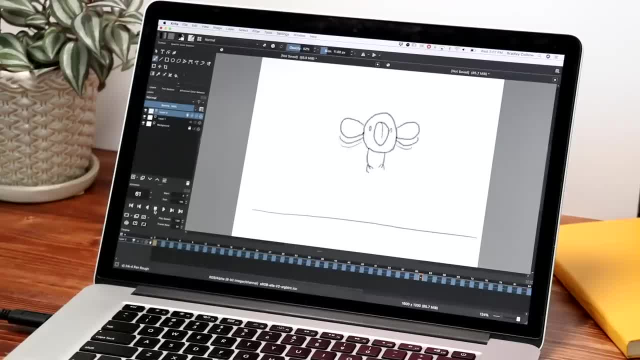 but you might get charged for it there. Just go to kritaorg And if you really love Krita and want to support what's going on over there and the development, there is a donation option available on their website. Speaking of websites, today's sponsor is 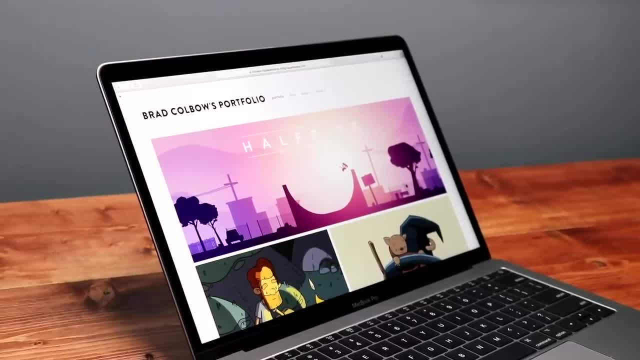 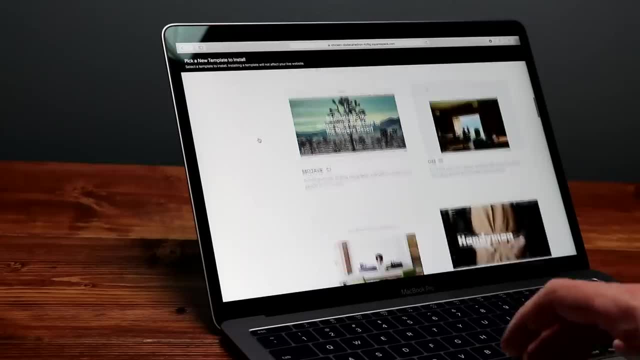 Kryta Squarespace can hook you up with one. I took it for a spin and built a portfolio to showcase my illustration work. They have some really nice templates. They're just easy to customize: Portfolio templates, e-commerce templates, blog templates- That's just scratching the surface. 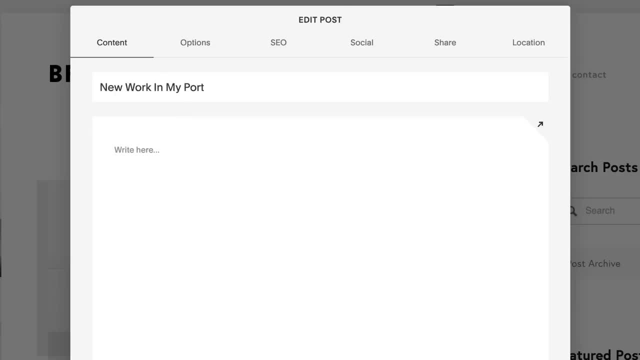 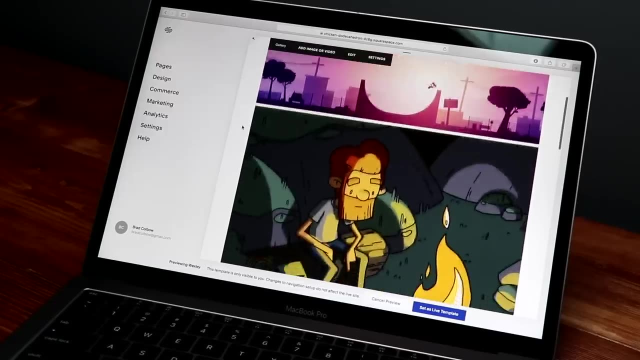 All of these templates are a great starting point for whatever you want to create And as a former web designer, I like the fiddle, So I like that I could jump in and get really granular with the design. If you're showing off your work to potential clients or you're looking. 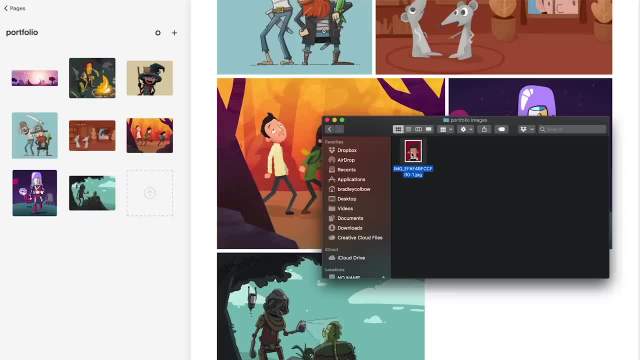 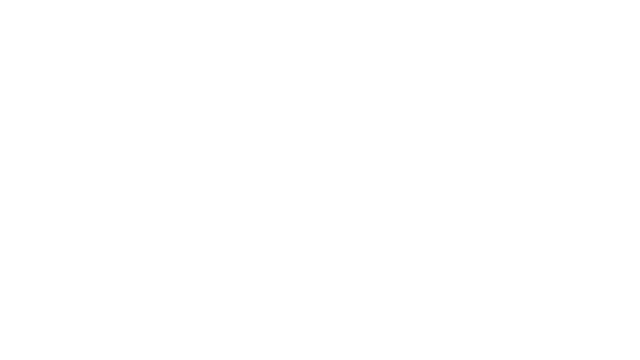 to land a full-time job. these templates look really professional And if you want to take your website to the next level, you can set up your own domain or transfer one you already have. Head to squarespacecom for a free trial And when you're ready to launch. 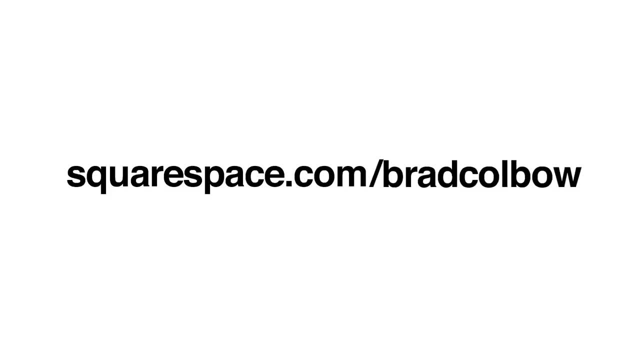 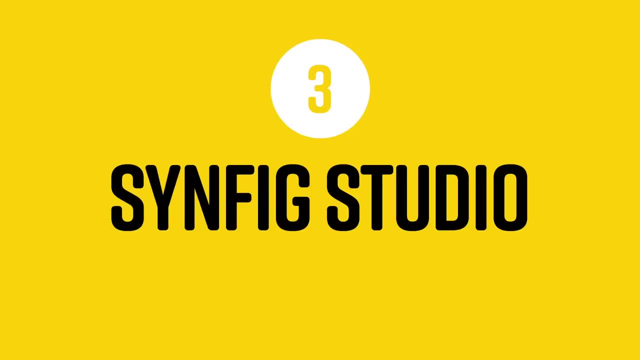 go to squarespacecom- slash bradkolbo to save 10% off your first purchase of a website or domain. Next on my list is Synfig Studio, and it can do everything I can do in Adobe Animate- At least on paper it can. That's the good news. 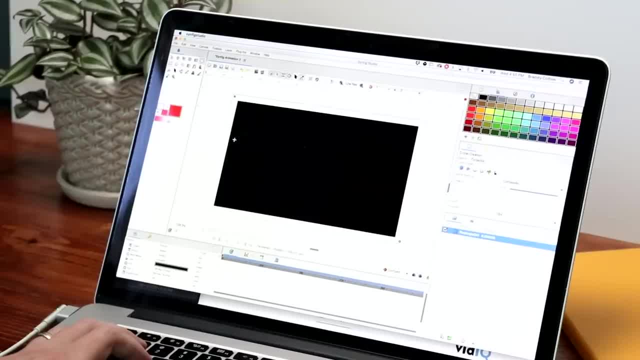 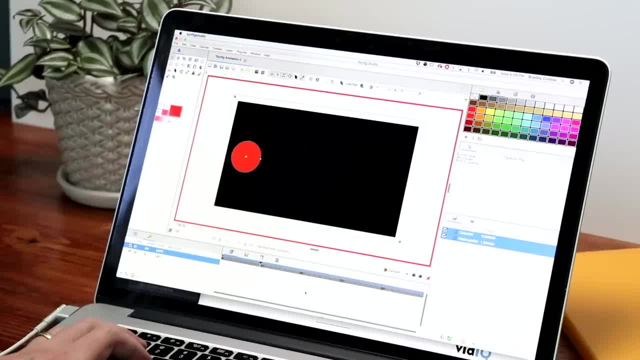 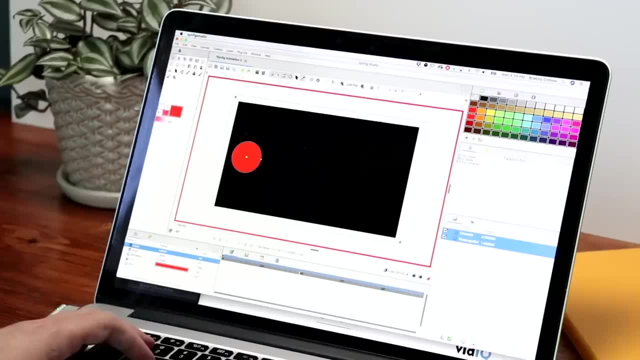 I felt pretty comfortable with just jumping in and doing some simple animations. Synfig did throw me a little. Maybe it threw me a lot. For example, it's pretty common for me, when I'm starting up with a new program, to Google how to do things. Usually, the things I'm Googling. 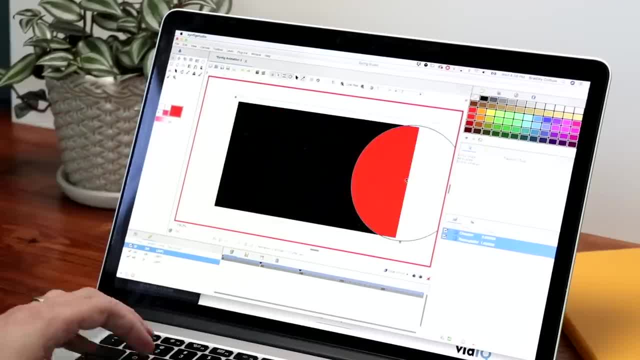 aren't like the obvious things, but here I had to Google everything. I had to Google. how do you delete something in Synfig. It's not as easy as just hitting the delete key. The upside is under the hood. Synfig can do so much. It really seems like it can do just. 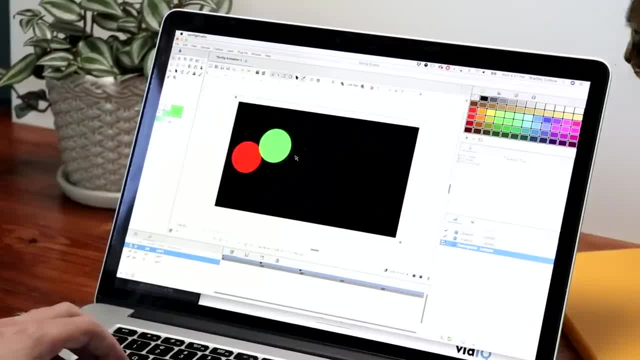 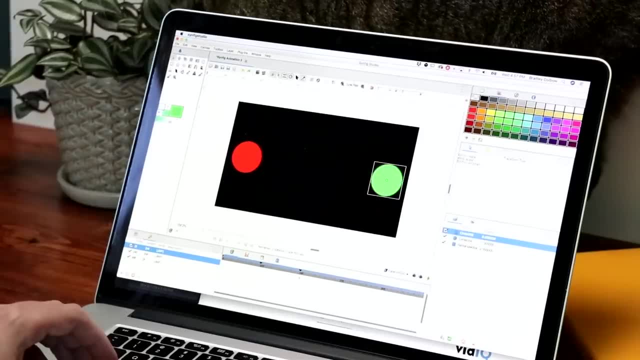 about anything here. I just have to poke around long enough to figure out how to do it. If you're going to tap the potential of this app, make sure you set aside a good chunk of time to actually learn it. I would also encourage you to make your own art assets in another app and then bring them. 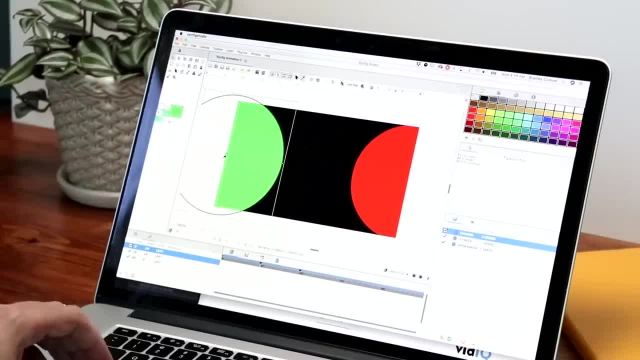 over. Synfig does have some basic drawing tools like brushes or razors, but they're not really good to draw with. Sometimes I like to draw fast and those strokes can get a little geometric. So, Brad, why the heck is this on your list? Well, I almost pulled Synfig off, but 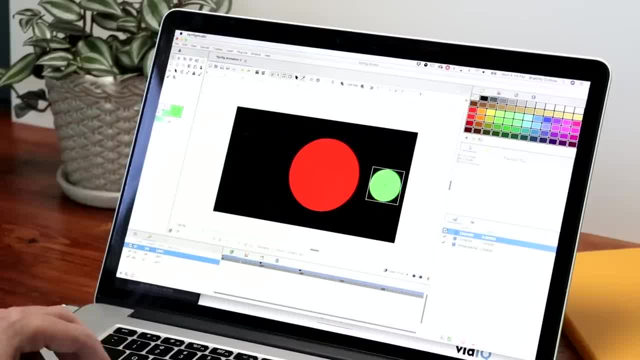 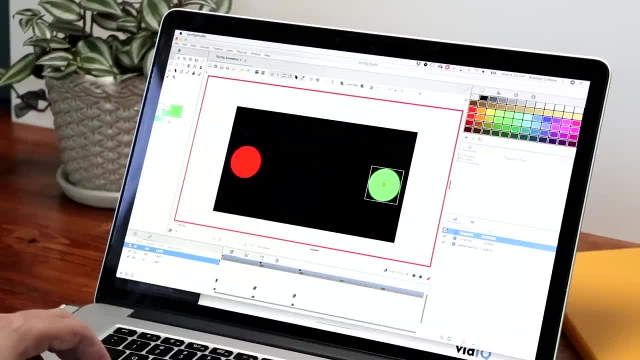 because of its support for tweening animation and some of the advanced rigging options for character models, I felt like it should really be here. I feel like there's a lot of folks out here who would truly appreciate everything you can do in this app, and it was worth sharing. 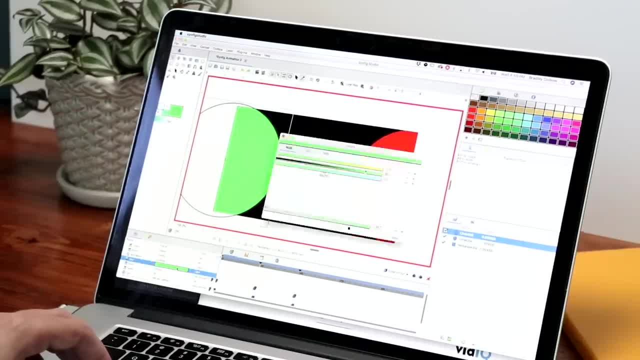 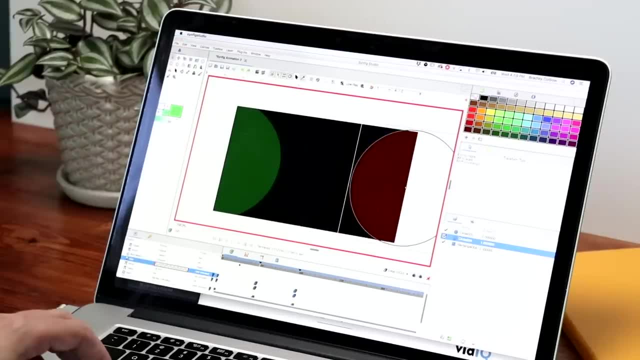 There are some really advanced features here that you just don't usually see in free apps. In fact, I think I can confidently say you can find in no other free app For complicated videos and animations. this can be very, very powerful, and I can't state that enough. 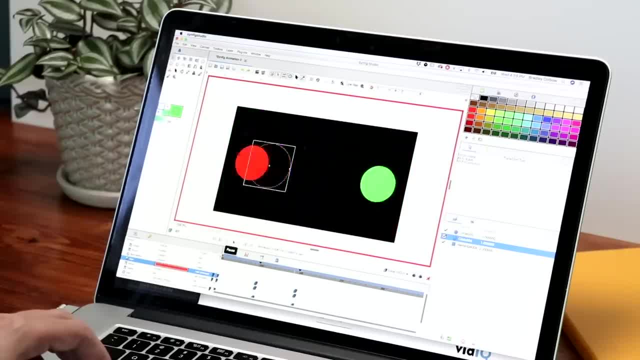 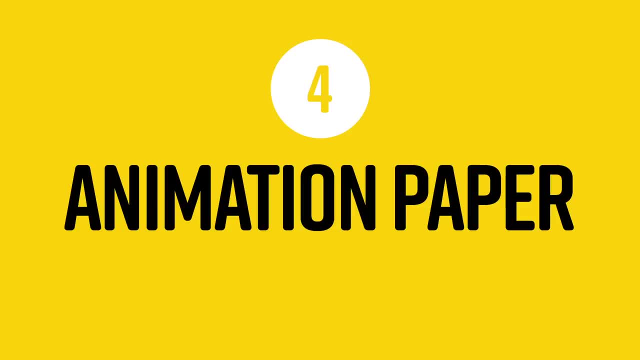 So Synfig gets to stay on the list. Just make sure you approach it with patience if you plan to get the most out of it. Next up, we have Animation Paper. It is developed by one guy whose name I am about to mispronounce: Niels Krog Mortensen. I have a soft spot in my heart. 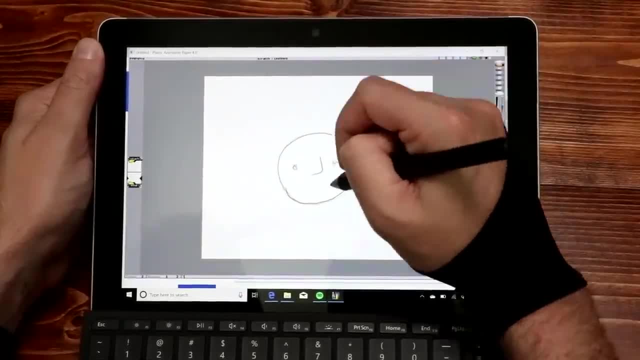 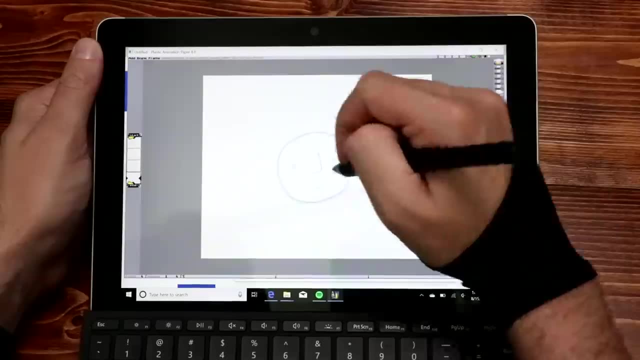 for software developers who are just out there making their own thing. That's exactly what he's doing Now. technically, this app doesn't fit all five of my criteria, but after watching him talk about why he's designing his animation app the way he is, I love it, man. I just had to add: 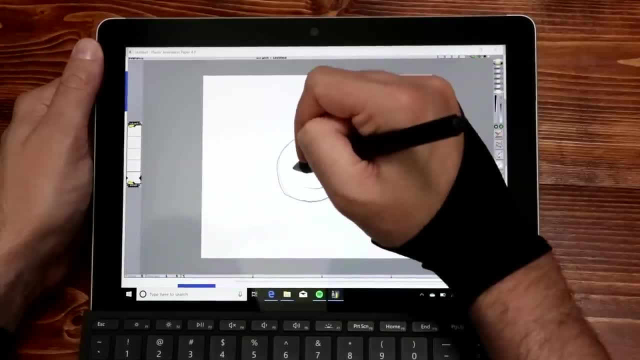 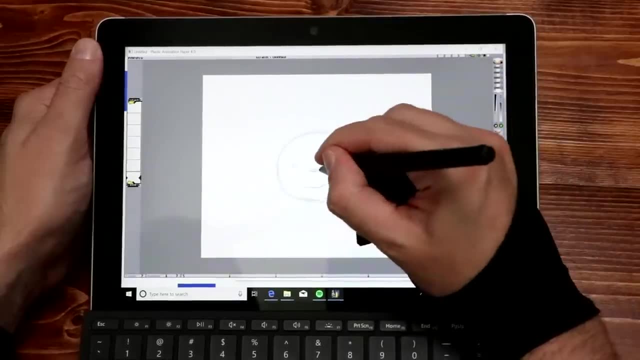 it to my list. Animation Paper is primarily a frame by frame animation app. Niels is a character animator and looking at how he uses his own app, it is really good And every feature in this app is in here. for a reason, There's a strong emphasis on flipping In traditional animation. you're 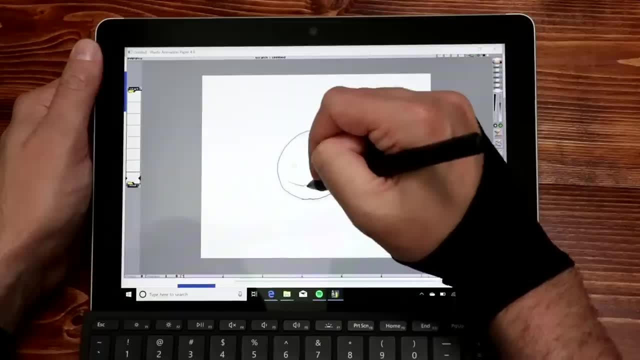 flipping the pages of your animation so you can see how they flow. He's built a lot of that into this app and it goes beyond just onion skidding. He's built a lot of that into this app and it goes beyond just onion skidding. He's built a lot of that into this app and it goes beyond just onion. 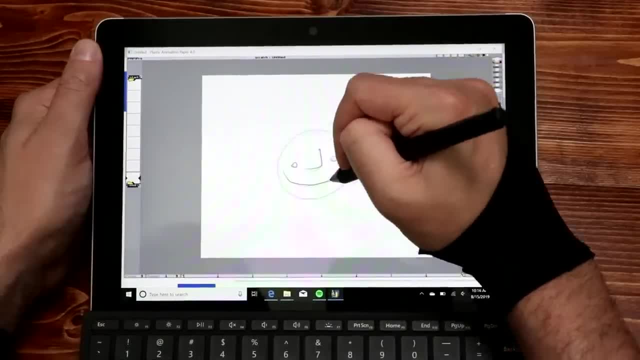 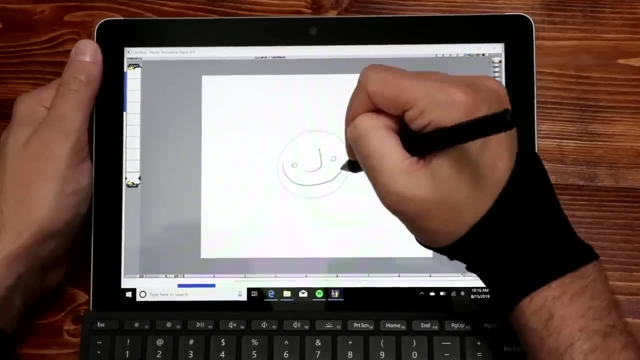 skidding. Responsiveness and smoothness of his previews are also a high priority because, in frame by frame animation, being able to preview your animation a couple frames at a time and see how smooth your animation is is a big, big deal. This app is built from the ground up. 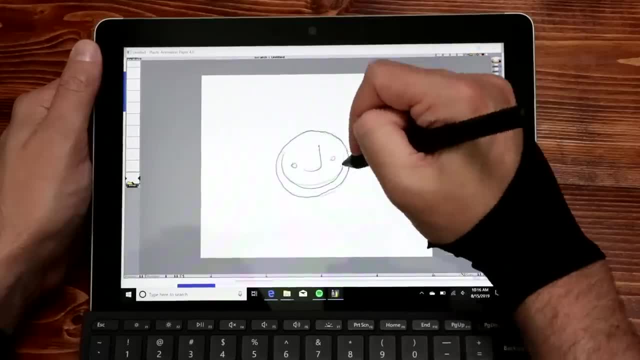 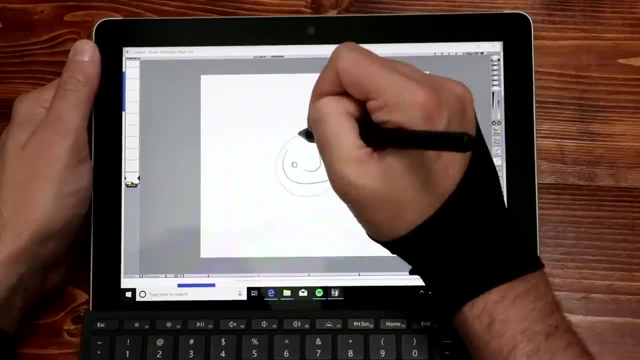 with that workflow in mind. He's not reinventing the wheel or doing anything I haven't seen in other apps. What makes this special is how he has chosen to prioritize the features. He is a professional animator and he uses this for his own workflow, Even though there's 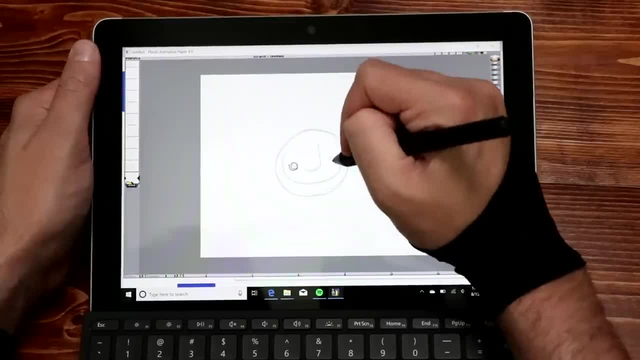 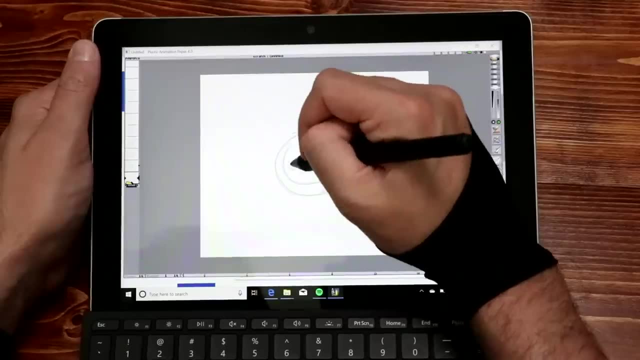 no tweening included here. he has other features in place that makes it really easy to duplicate multiple frames at a time. So say you make your character's animation walk cycle. you can repeat that over and over again without doing a lot of extra work or heavy lifting. Same with tools that. 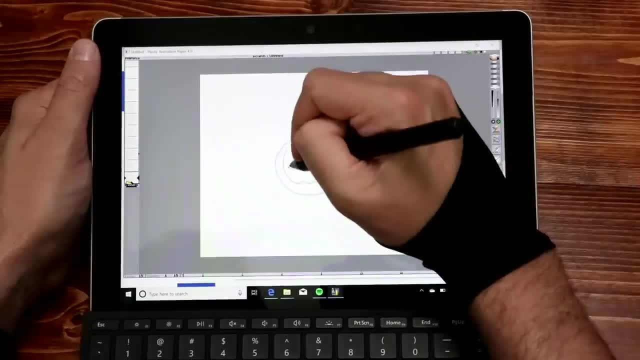 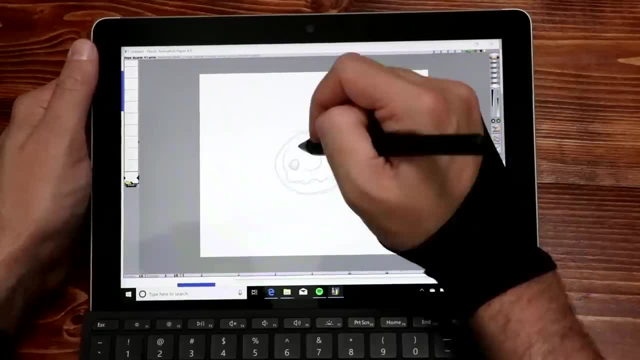 allow you to duplicate portions of your artwork that you can reuse on other frames. These aren't symbols- necessarily like the way Adobe Animate has symbols, but they can function and you can use them in a similar way, And because of that, it feels like it makes the process a lot easier. 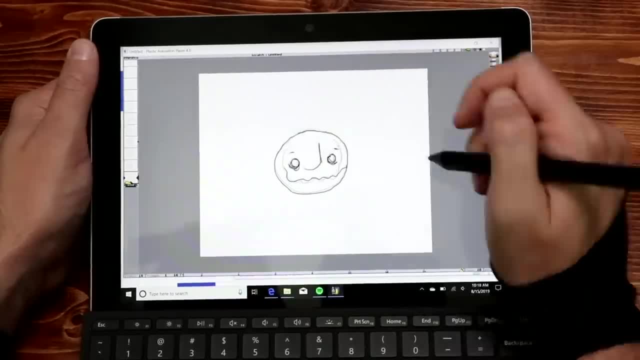 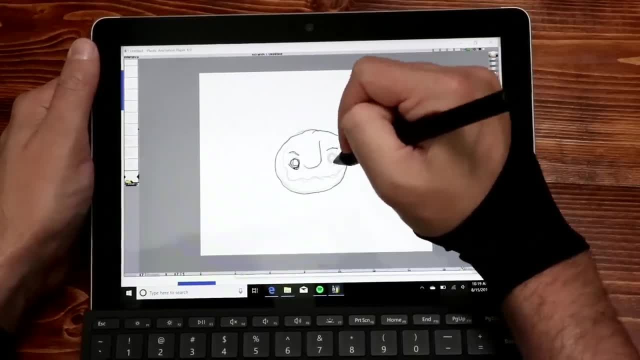 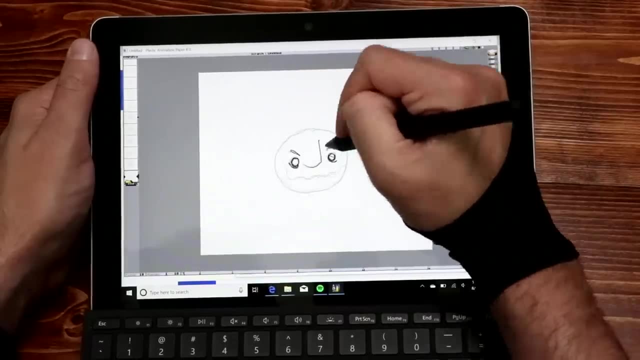 There's an ability to leave notes next to your frames. I can see here in his own samples he has notes on how long he wants each part to take, kind of the bouncing of his animation cycle. I had never thought of that, but being able to kind of map out your animation ahead of time to 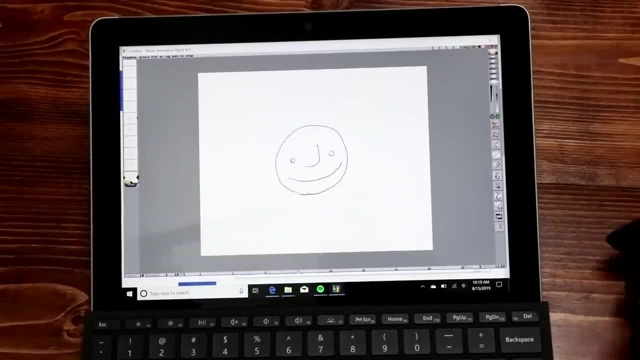 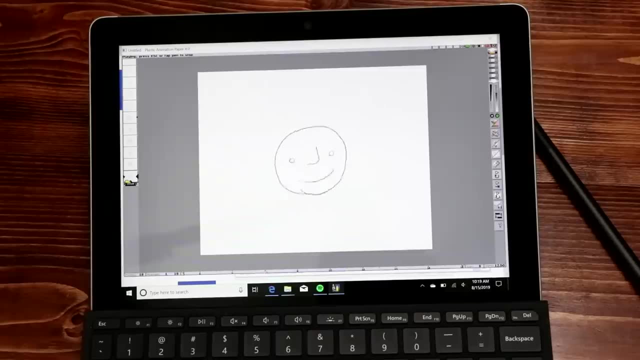 know how long it is, could be incredibly helpful. He's also working on a new version of the app. He's charging for beta access to that, but right now the Windows version of the old app is completely free and available on his website. Last but definitely not least is OpenToonz. 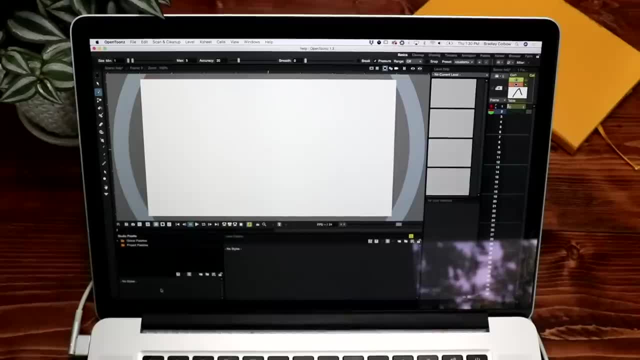 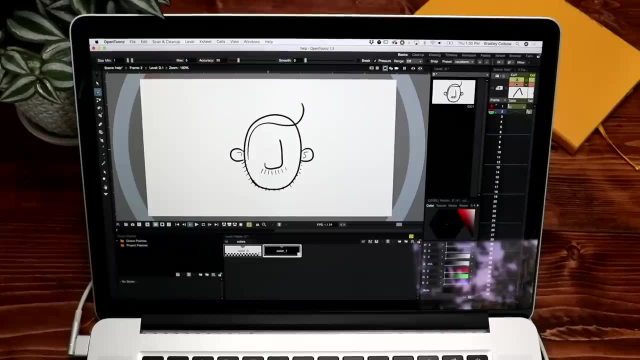 which is probably my winner for checking the most boxes and coming the farthest to replace Adobe Animate for me. In fact, if I had to, I could replace Animate completely, just with OpenToonz. It does everything I need it to do. In fact, it does a lot, lot, lot more. 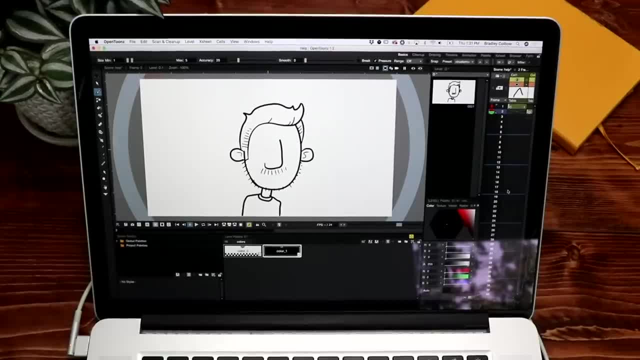 If we start by looking at the drawing tools, they're just far beyond what you're going to find in Animate. Well, they kind of are In base OpenToonz. they're not, but you can add to them. For example, you can add in my paint brush sets into OpenToonz, and there are a lot. 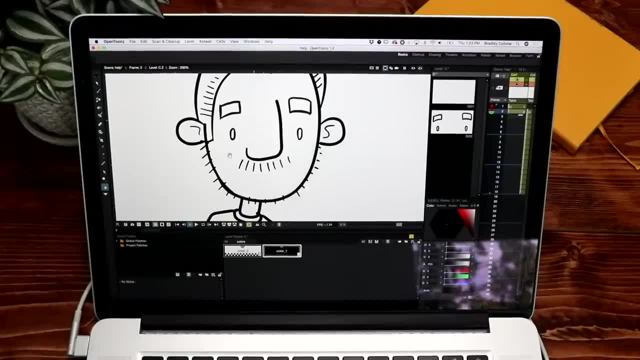 of cool natural media brushes here that can turn OpenToonz into a full blown art app- Maybe not quite on the same level as Krita, but it's a big step closer to it. On top of that- the native OpenToonz- you can have vector paint brush options, So if you want to sketch with, 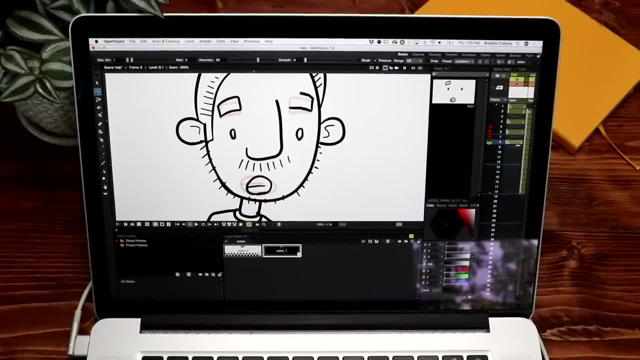 say a pencil, and then finish it off with brush and inks done in vectors. you can totally do that here. If you're used to using Adobe Animate, I will say this is a very different program and a lot of the differences are in how things are labeled. 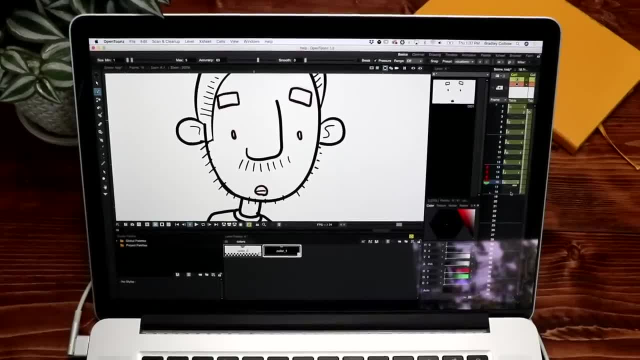 and how the workflow is handled. For example, symbols are called sub sheets. Took me a while to figure that one out. One piece of advice that I saw over and over again in my research were folks saying: don't treat this the way you treat Adobe Animate. Instead, treat it like its own thing. 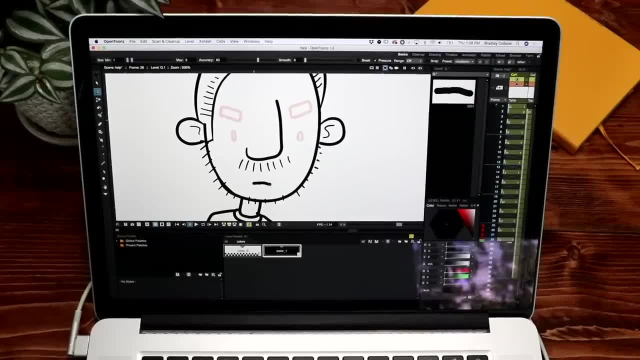 OpenToonz is built around the way traditional animation studios work and it pulls a lot of its vernacular into the application. Instead of a horizontal timeline, you get a column view of the animation. At first I found this really disorienting, but really it's not bad, It's just. 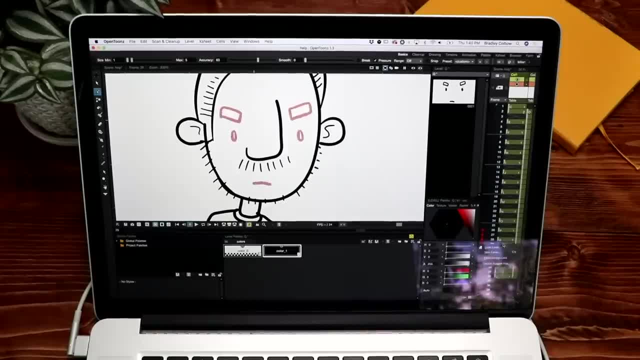 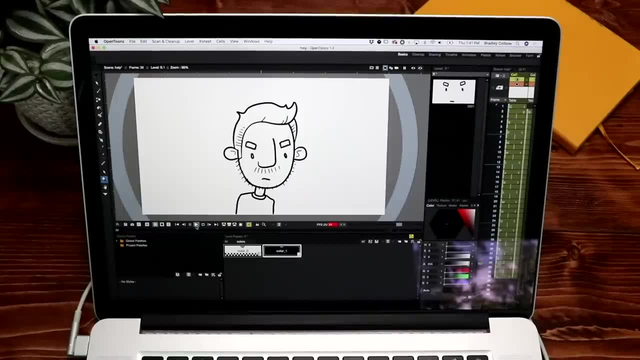 a little different. Overall, I feel like I've barely scratched the surface of what OpenToonz can do. There's a whole camera system that I don't fully understand how much it can do. There's a whole FX schematic section which I completely don't understand what you can do. 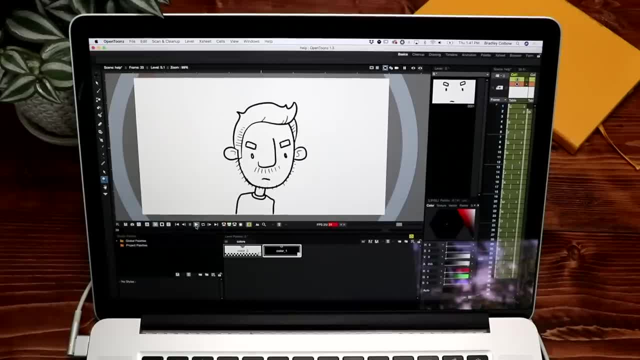 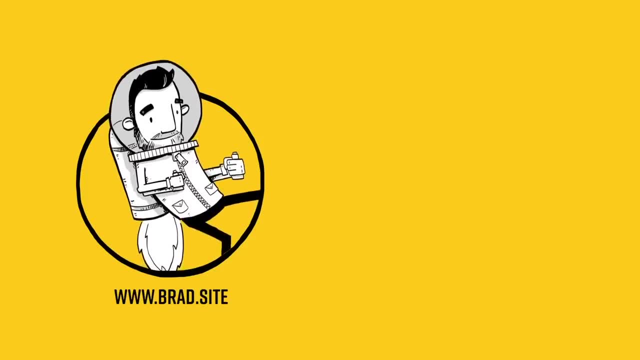 There's just so much here, And you can grab OpenToonz on their website, and it's available for Mac or for Windows. So those are my five favorite animation apps. What is your favorite? Did I leave it off the list? Let me know. 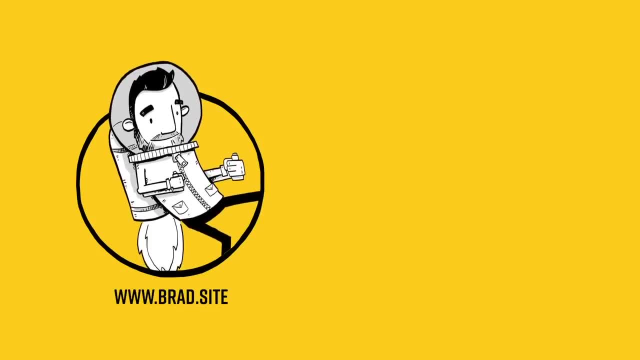 And down below in the comments. thank you guys for watching, Really appreciate it And I'll talk to you in a couple of days. 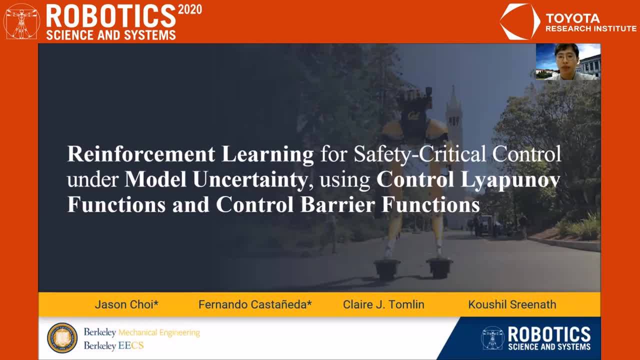 Hello, my name is Jason and in this video I will be talking about our paper Main Persimmon: Learning for Safety: Critical Control under Model Uncertainty, Using Control-Yakono Functions and Control-Bearer Functions. Model uncertainty is present in all kinds of systems, from ground and aerial vehicles to